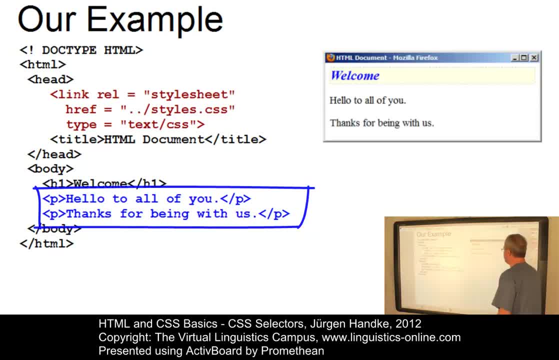 in its body, resulting in two paragraphs in the browser. This allows us to show the effects of style changes more appropriately. Since we are now using an external stylesheet, we do not have to present the HTML code any longer, but just the content of the external stylesheet and the changes made within it. 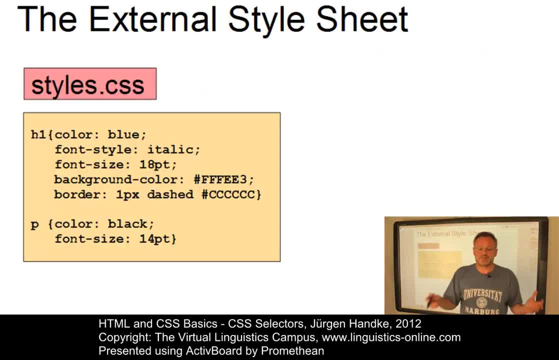 So here is our external stylesheet. Its file name is styles and its extension is CSS. Currently, this stylesheet contains two selectors with several property value pairs. They affect the H1, that is, heading level 1- tag and the P tags. 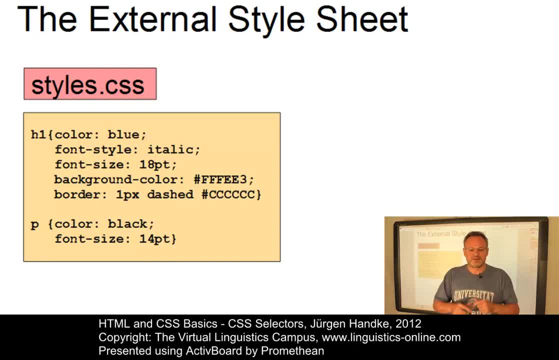 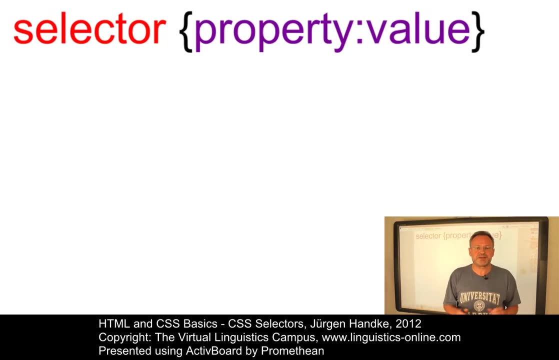 Before we look at the selectors that are possible within a cascading stylesheet, let us provide an overview of the use of selectors first. Now, the selector is the element of the style sheet. It is the element of the style sheet. It is the element in a CSS rule which identifies the HTML element to which a rule applies. 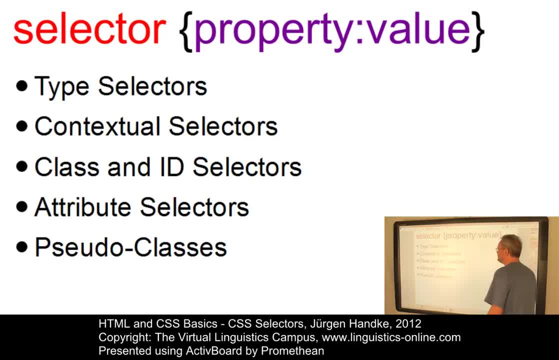 The following selector types will be discussed in this e-lecture. We will first look at type selectors, which redefine HTML tags. We will deal with contextual selectors, We will look at class and ID selectors and at attribute selectors And finally we will deal with so-called pseudo-classes. 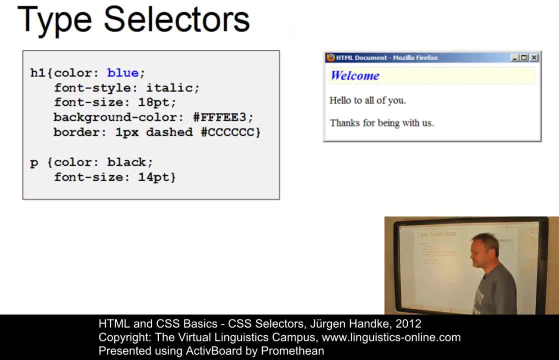 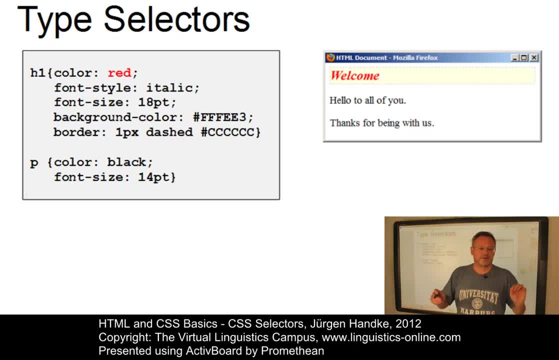 Let us change one of them And define the heading now in red And, as you can see, a simple re-declaration of the color property of the H1 selector in the stylesheet will do the job. Contextual selectors are contained within another selector. 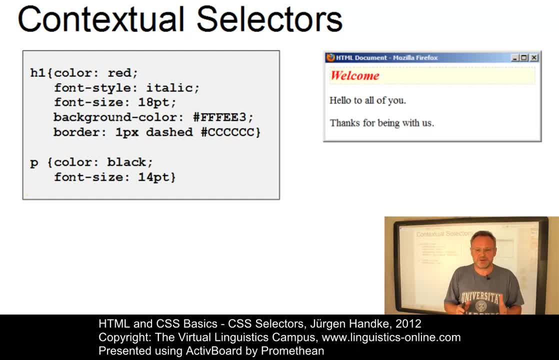 They are indicated in a list separated by a character. They are indicated in a list separated by a character, character, space, starting with the higher level element. Here is an example: An emphasis selector applied to the paragraph tag. It assigns the color green. 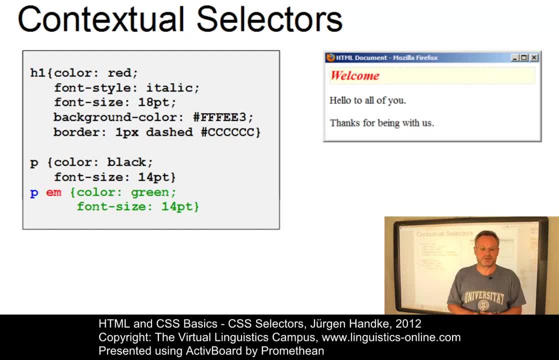 to all emphasis tags within all paragraph tags. To see the effect, we have to change the HTML document in this particular way. Now we inserted the emphasis tag into the paragraph tag and the result is what we would have expected. The string all of you is now green. The remaining strings within p tags. 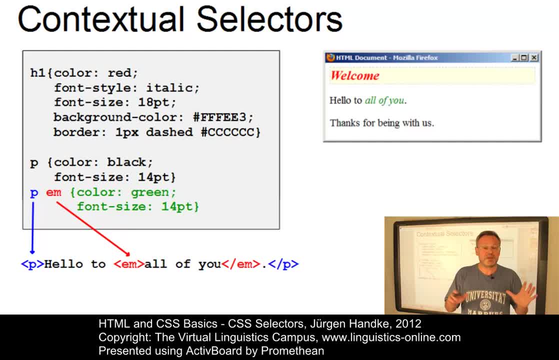 and all other emphasize tags will remain green. So our new style definition only applies to certain contexts. Let's look at class selectors next. Class selectors are used to apply a style to a special kind of one or more HTML elements. They can be used to mark: 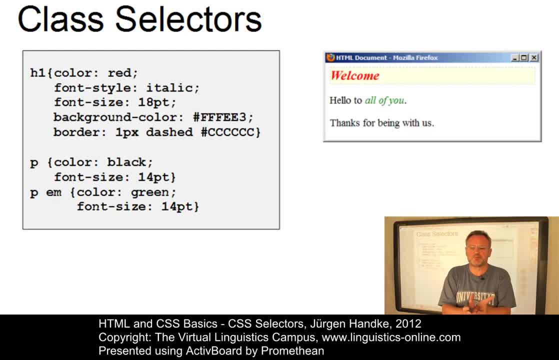 elements which belong to a conceptual group. This means that not all paragraph tags are changed, but only those paragraph tags which have been given a special attribute. Here is an example. Now pspecial- and that's a syntax- is now our new selector. It is written in the dot: syntax Type selector. 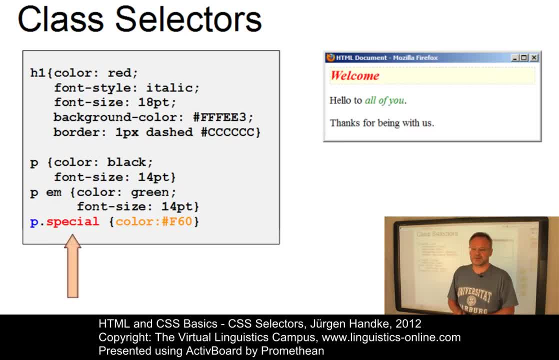 dot class selector. and then of course, the property value declaration. Here we would define the color orange to particular paragraphs In the HTML code. we can now add the attribute class with the value special. As a result, this particular p tag displays the text in an orange color. 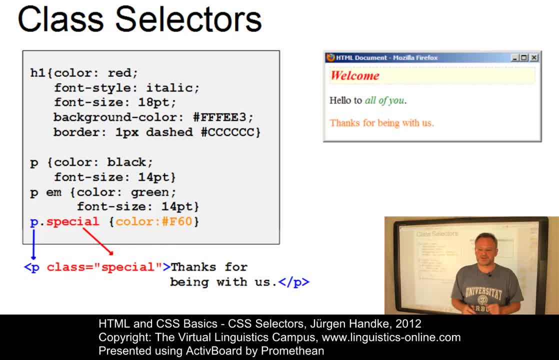 In our case, only p tags which have been given the class attribute special are displayed in the respective color. If you want to apply the rule to other elements, it is possible to leave out the HTML tag, thus making it possible to apply the rule to other tags. 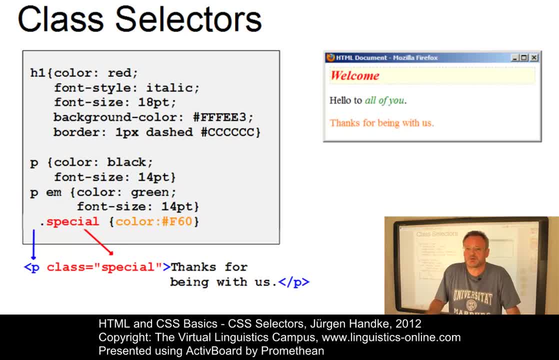 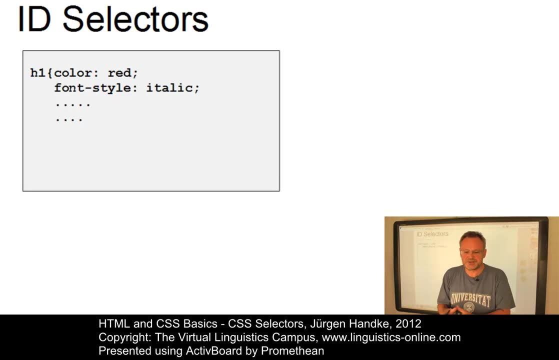 with the class attribute special, For example. we could define headings in such a way. Let's now look at the ID selector. The ID selector is used similarly to the class selector, with the only difference that the respective element can be used only once within the HTML document. 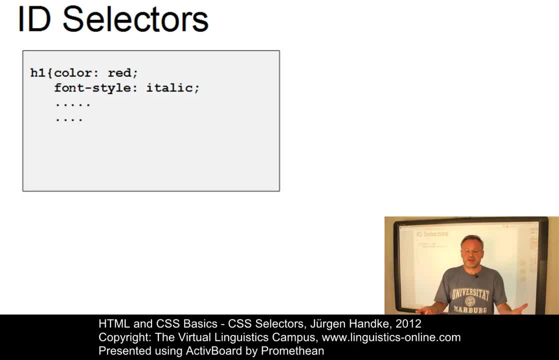 This results in the fact that IDs can be used to mark elements semantically, That is, the ID value should be a self-explanatory label for the element In the style sheet. ID selectors are presented as follows. They are introduced by the type selector. Here it is. 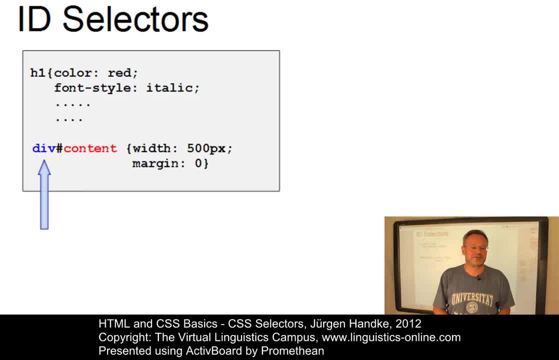 a division type selector. Then they're followed by a hash tag, and then the ID selector, that is the self-explanatory label we assign to them, And then, of course, the property value list. In this case, the div tag would be defined. 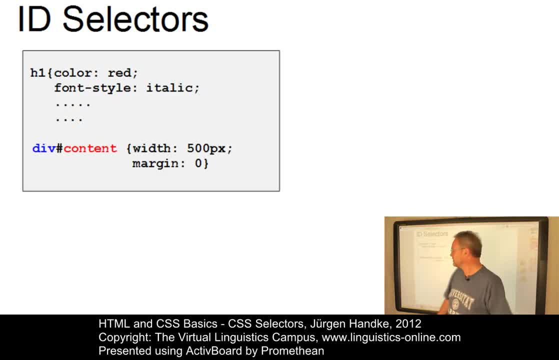 with the width of 500 pixels In the HTML code. we can now supplement the target tag, that is, in our case, the division tag, with the ID attribute and the value of the name we defined earlier on. The value, of course, has to occur in quotes. 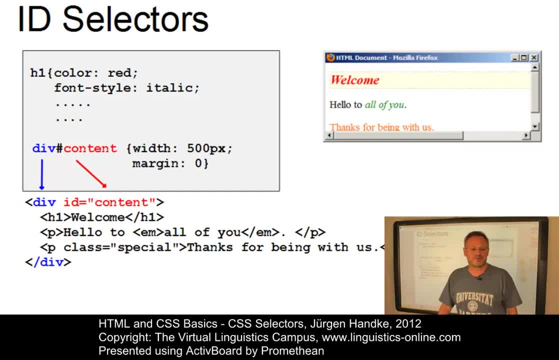 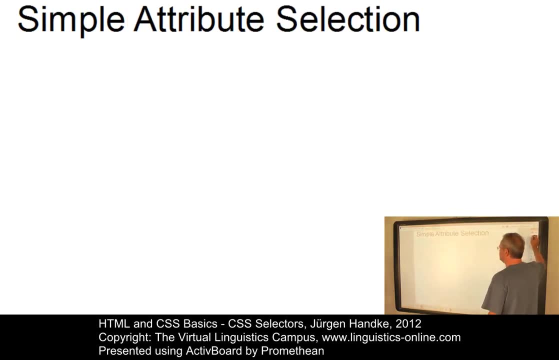 In our case, the effect that we can see in the browser is not very convincing. The width of 500 pixels leads to the occurrence of scroll bars in our small browser window, but it shows that the ID selector works. Let's next look at attribute selectors. 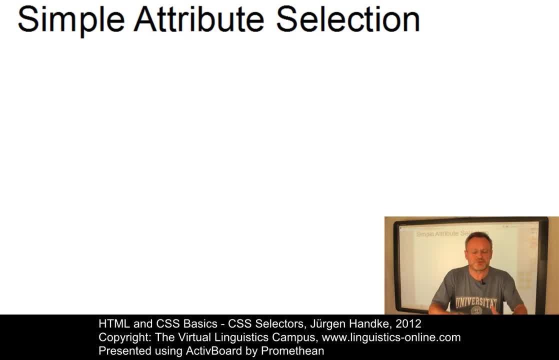 Now, attribute selectors, as you can see, are very useful. Attribute selectors affect the attributes of HTML tags. This is useful when you want to address tags which do not contain any class or ID attributes. Attribute selectors have the following syntax within the style sheet: 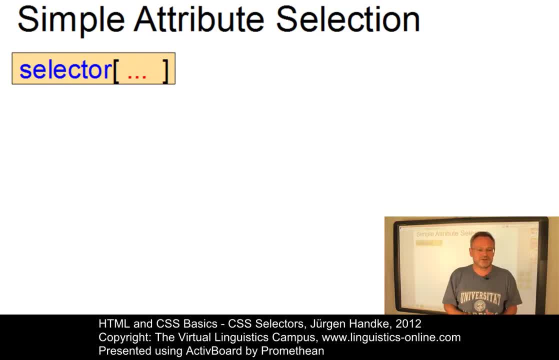 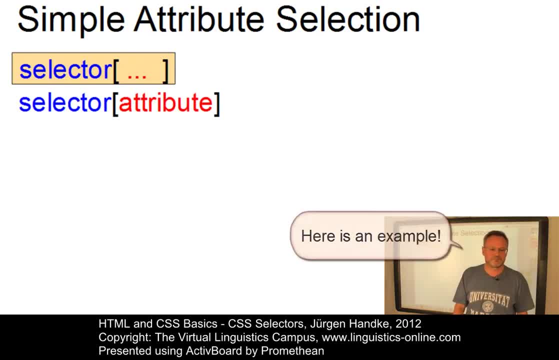 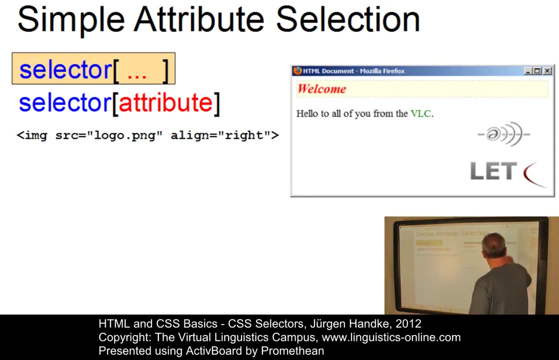 Here is an example, the so-called simple attribute. In a previous version of our HTML document, we had an image using this image tag in the body, And the result was that the VLC logo and the LAT logo as one image were aligned on the right-hand side in our web document. The file name is logopng. 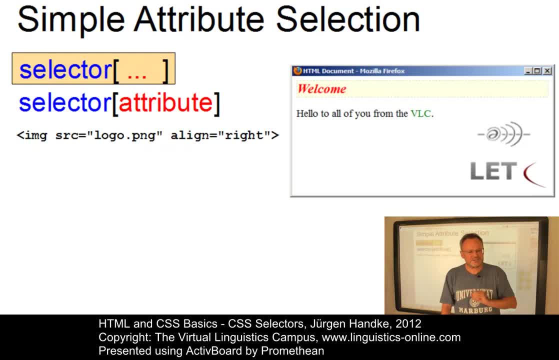 The file name is logopng. Let us now assume we have several images on our website which we all want to frame red. All we have to do is use the title attribute within the image tag of the images which we want to frame and we have to give to the title. 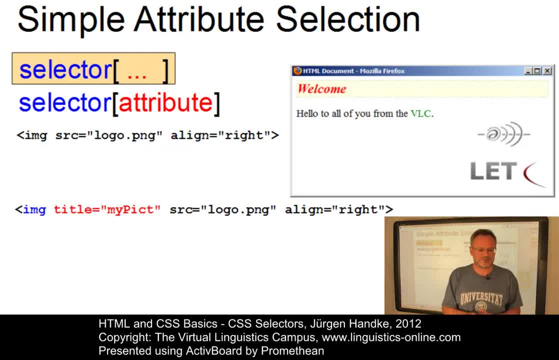 attribute as a value, a name of our choice. In the style sheet the rule looks like this: It references or selects all images with a title attribute and any title value. They only have to have a title attribute And it assigns the predefined properties to them. 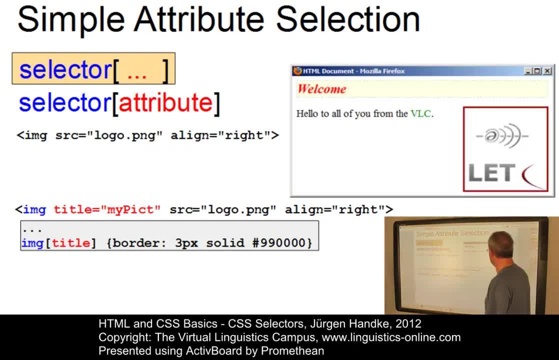 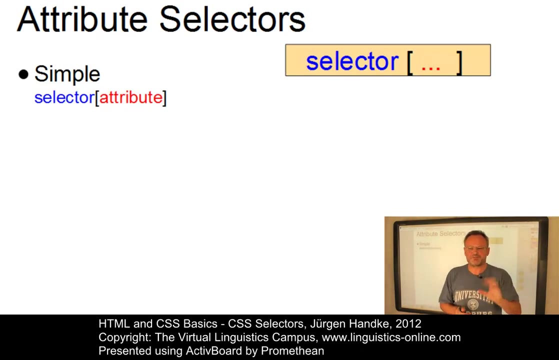 The result in the browser is this: A frame around our picture becomes a title Because it is associated. the image tag is associated with the title attribute and a name given to it. There are several ways of attribute selection, but since browser support is a bit disappointing here, 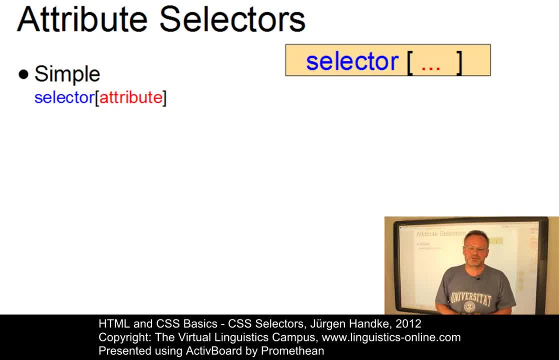 we will just list them. The simple way of attribute selection has just been demonstrated. The simple attribute selection, The exact way of using attribute selectors, references only those elements whose attribute not only matches the style property but also its value. so these, these strings have to be identical. the partial method references those elements. 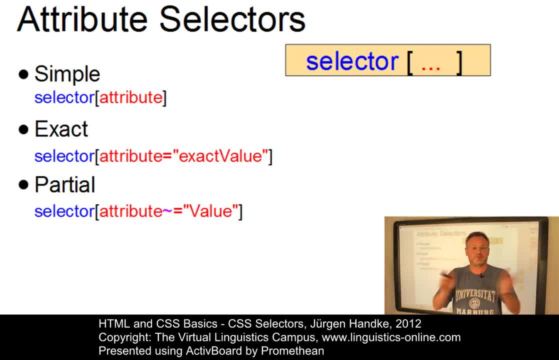 where the tag attribute and the style property match and the property value is contained as a substring in the attribute value. and then we have the hyphen separated form, which is very similar to the partial form. however, here the property value is a sequence that involves a hyphen in the attribute value. 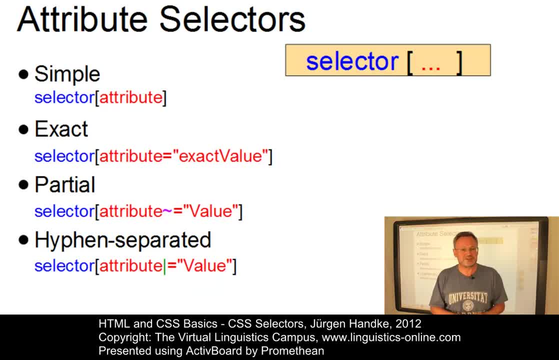 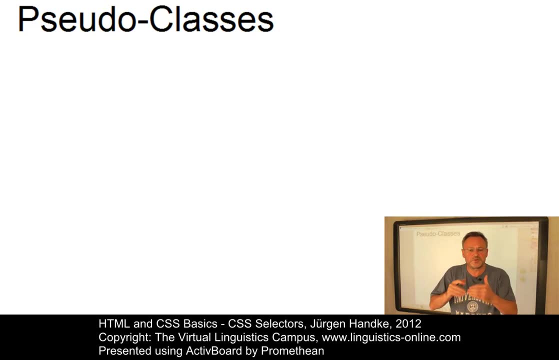 further details can be found in the VLC virtual session: cascading style sheet layout principles. so let's continue with the another class, with the so-called pseudo class. now, pseudo classes are based on the state of an HTML element or the document itself. the most common use of 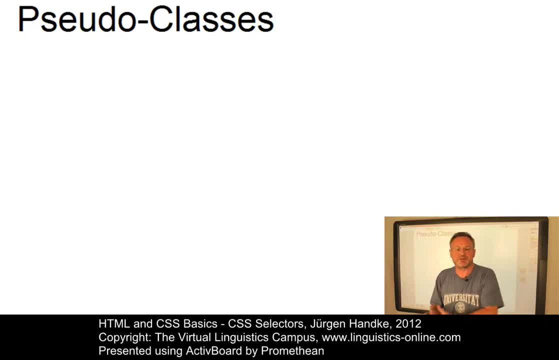 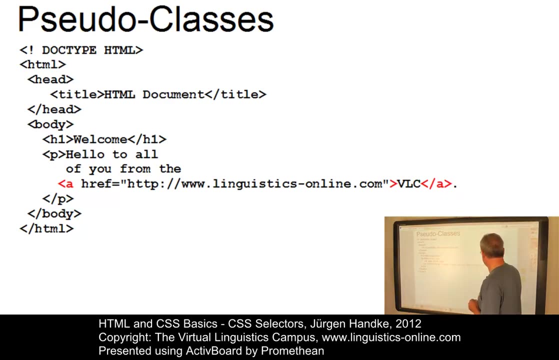 pseudo classes occurs when a certain state of a hyperlink is triggered by the user. so let us use our standard code again with hyperlink anchor tags around the item VLC over here. by default, the browser underlines the hyperlink and displays it in blue with the anchor tag pseudo class. however, we can address the various states for. 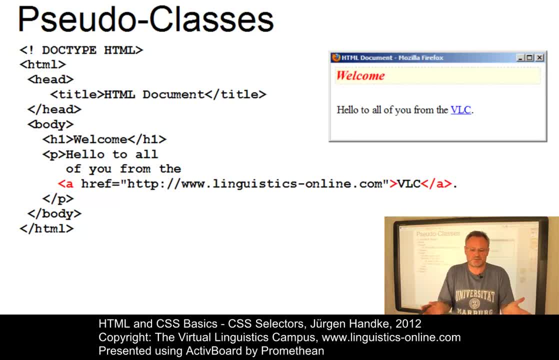 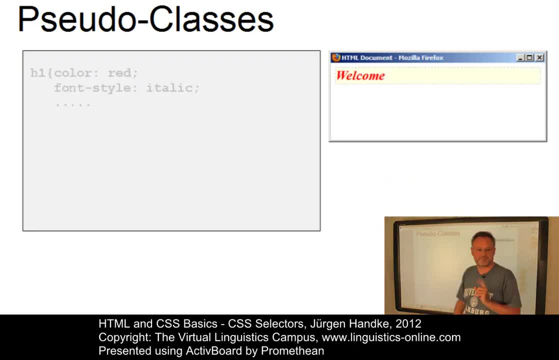 hyperlinks and assign different colors and text decoration to them. so let's show how this is done. with the pseudo class anchor colon, link, anchor colon and link, we can define the state of the link itself, that is, its default value. in this case, we are overwriting the underline. 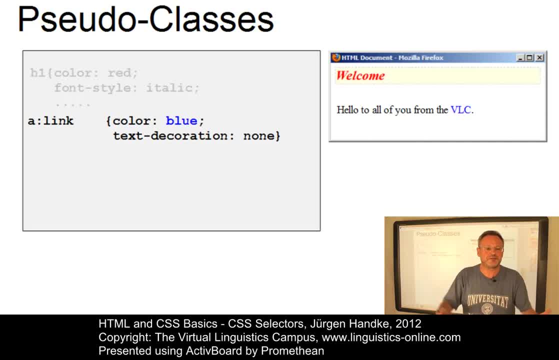 definition by the browser style and are defining the new style. no further text decoration, the, the. I don't want to go too far into detail here, so let's take a look at some of the pseudo classes that are used in the style sheet, and we simply use the color black. 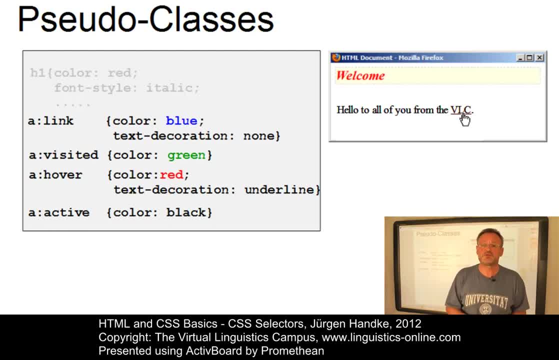 here. these pseudo classes can be used to increase the usability of an HTML document by giving feedback for user action. their sequence of occurrence in the style sheet has to be followed in order to let the effect work properly. changing the sequence will result in the prevention of these effects, so do not change this sequence here. 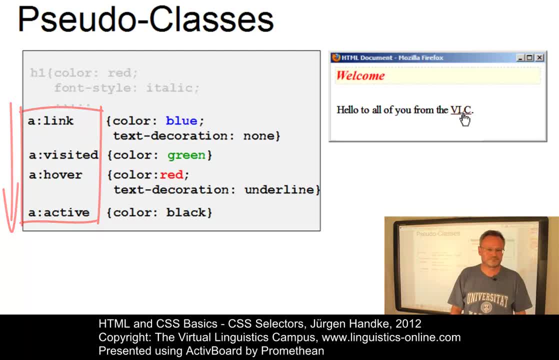 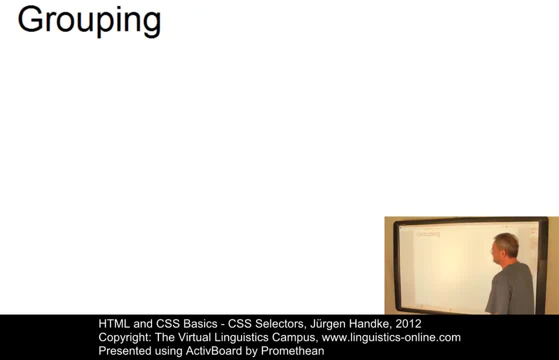 okay. now the final thing we have to discuss is the topic of grouping. now, CSS declarations can be grouped to apply one attribute to several HTML elements. this cleans up your CSS code and arranges things more clearly and improves readability. selectors can be grouped by listing them in front of their declaration, separated. 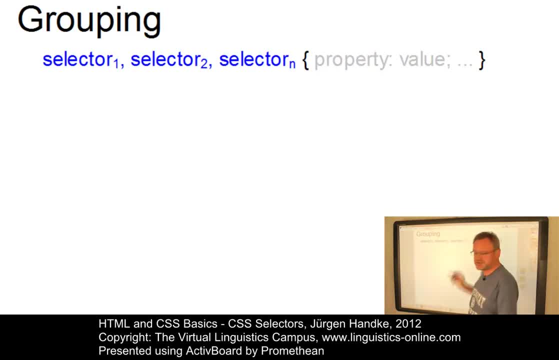 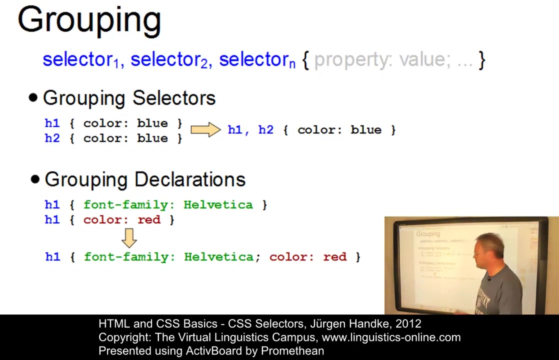 with commerce. here is an example which defines all types of headlines, while we are just using h1 and H2 tags here. so this example defines all headlines in blue. ok, ok, ok, ok, ok. We have already seen that we can group property value declarations Instead of writing one rule per declaration. they can be defined as one rule.